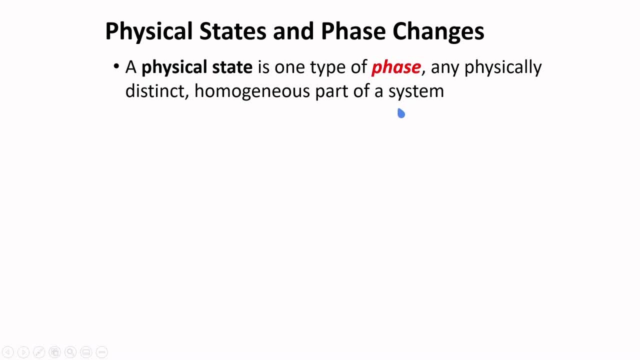 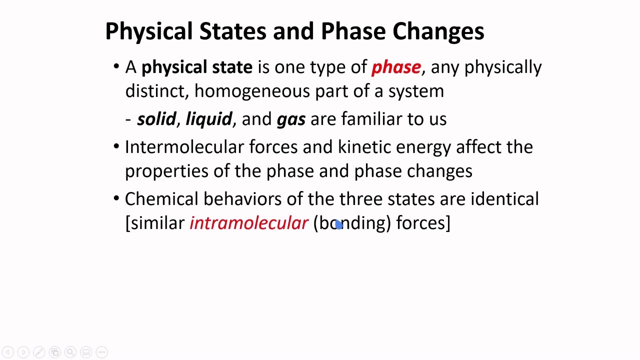 do not mix. Hence their mixture would be considered to have two properties: Solid liquid and gas are familiar to us. Intermolecular forces and kinetic energy affect the properties of the phase and phase changes. Chemical behavior of the three states are identical, That is, they have similar. 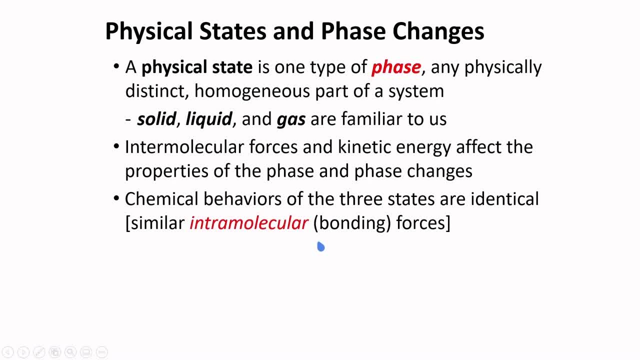 links: ofoto dehiers sequel: stark events. The bands that connect the atoms are the same regardless of states, Physical behaviors of the better. You are making your position unpopular. again and again, You are making your positionTSan танETuzang right. 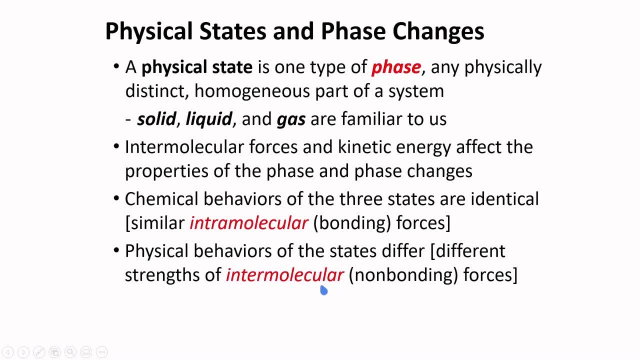 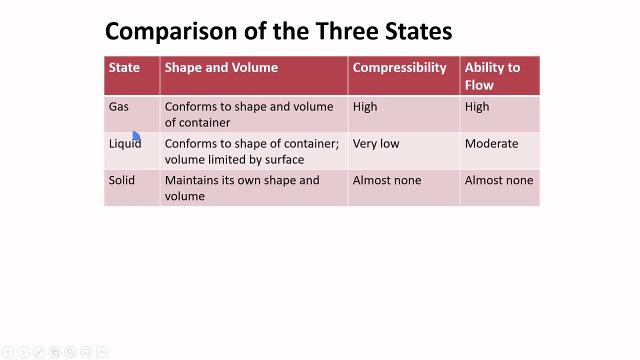 physical behaviors of the states differ. Different strengths of intermolecular forces are present are not the same as the strength of the intermolecular forces involved in gases. Here are comparisons of the three states of matter. The gas conforms to the shape and volume of the container. They are highly compressible and has a high 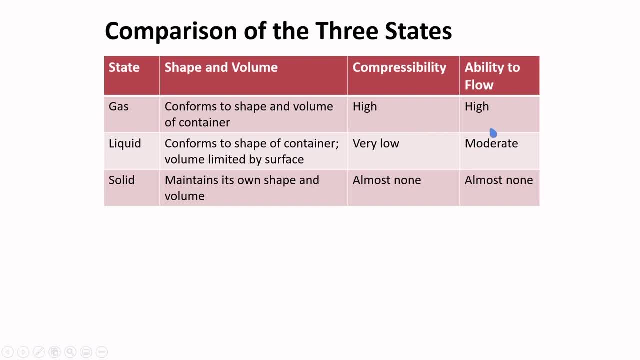 ability to flow. Liquids conform to the shape of the container and the volume is limited by the surface. Their compressibility is very low and their ability to flow is moderate compared to the gas. For the solid, they maintain their own shape and volume. They are almost incompressible and 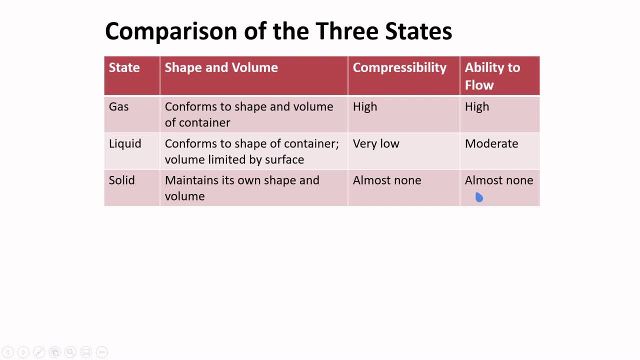 almost non-compressible. Almost no ability to flow can be observed. We can say that solids and liquids are condensed states. Liquids and gases are fluids. They easily flow compared to solids. The intermolecular attractions in liquids and solids are stronger compared to gases. 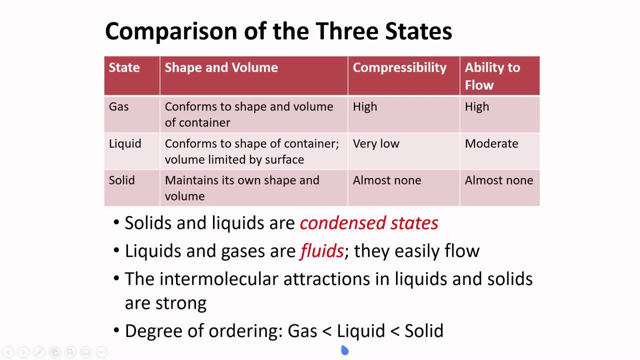 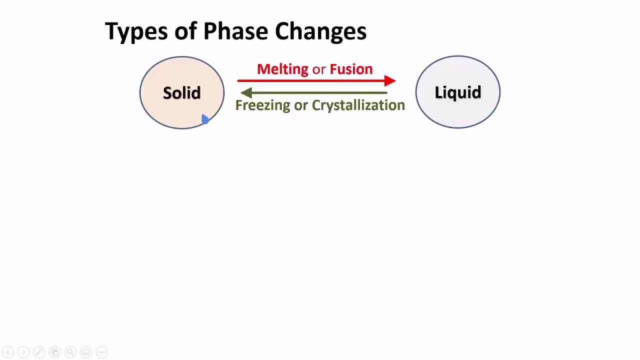 And particles of solids has the highest degree of ordering. There is a decrease in ordering, moving to liquid and then to gas. The different types of phases can interconvert. we can call the conversion of a solid to liquid as melting or fusion. Liquid can crystallize or freeze to form solids. 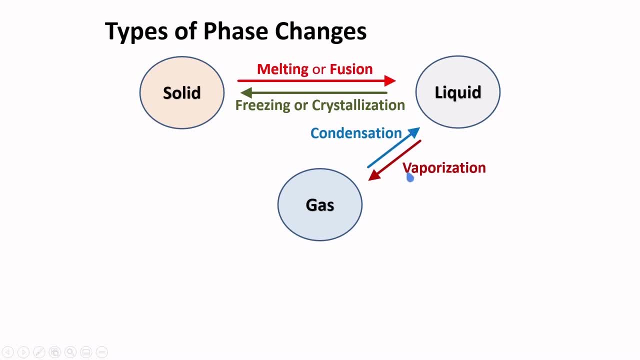 Gas can condense to a liquid and liquid can vaporize to gas. Similarly, solids can sublime to gas and gas can deposit into solids. Take note that condensing and freezing are exothermic changes. For example, liquid particles loses energy as they become solids. 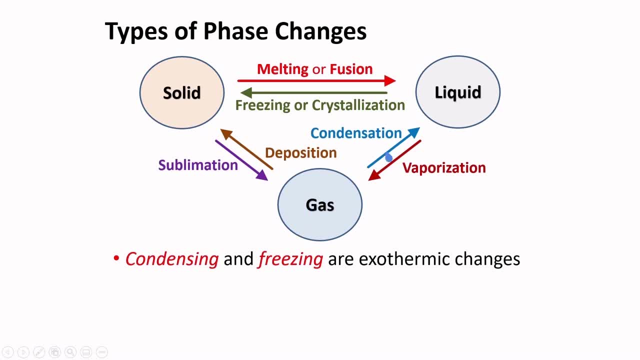 The same way, when gas particles condense to liquids, Thermal energy present in the particles are lost to the environment. The reverse of these processes- melting and vaporizing- are endothermic changes. You need to infuse a certain amount of heat in order for a solid to melt. Heating is required to convert a liquid. 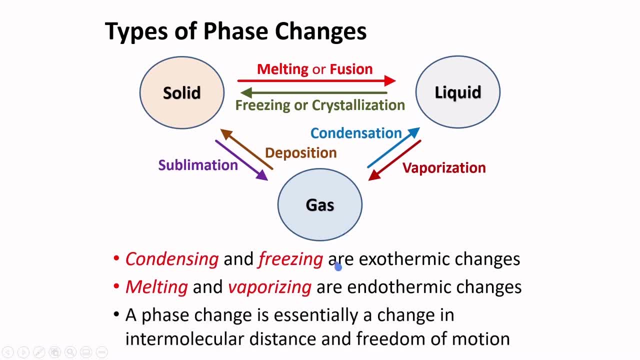 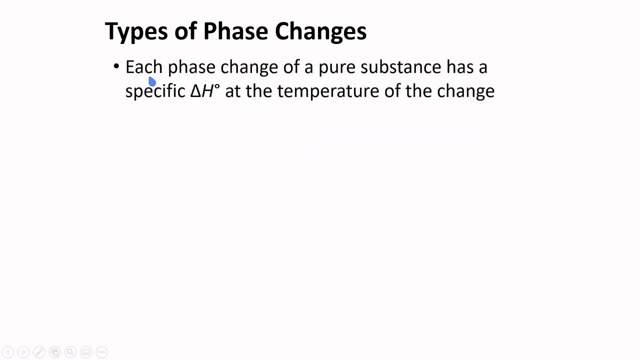 to gas. Overall, a phase change is essentially a change in intermolecular distance and freedom of motion. Each phase change of a pure substance has a specific enthalpy change at the temperature of the change. Opposing processes have the same magnitude of enthalpy change but opposite signs. 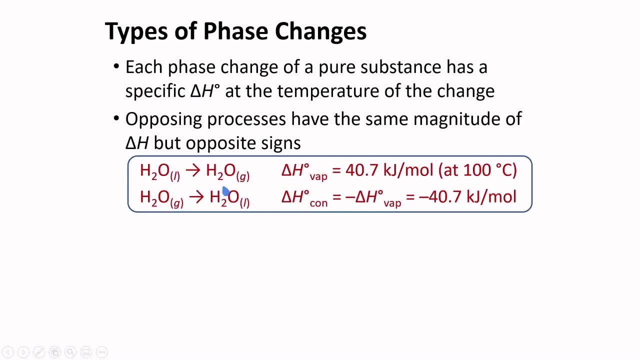 Consider the conversion of liquid water to gas. The heat of vaporization is about 40.7 kJ per mole at 100°C. If the reverse process occurs, that is, water vapor is converted to liquid, the heat of condensation is just the opposite sign of the heat of 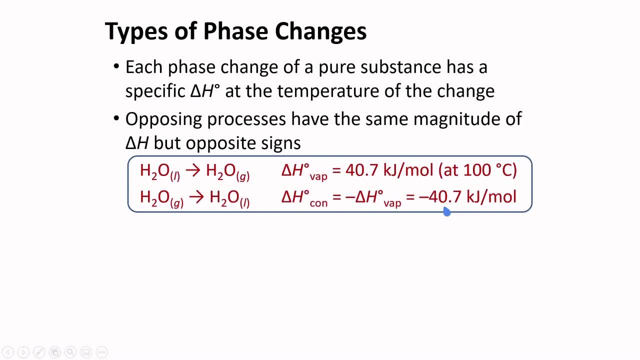 vaporization negative 40.7 kJ per mole. Usually it takes less energy to melt the solid form than to vaporize the same mass of the liquid form. The molar heat of fusion of water is 6.02 kJ per mole at 0°C. This is significantly. 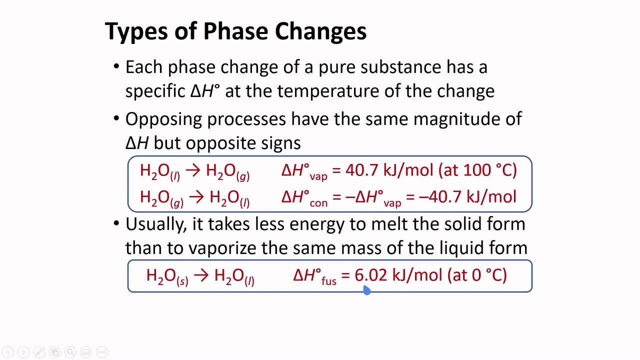 lower than the molar heat of vaporization. The difference in these values tell us that the conversion of liquid to gas for a certain material requires more energy than the conversion of the solid material to liquid. The heat of sublimation can be calculated from the molar heat of fusion and molar heat. 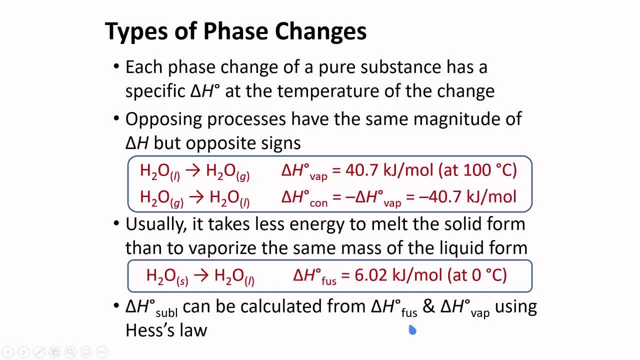 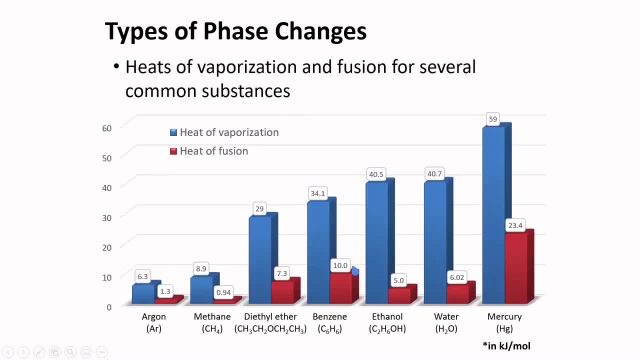 of vaporization using the Hess's law: Sublimation, Sublimation, Sublimation, Sublimation, Sublimation. Here are the heats of vaporization and fusion for several common substances. Not only does this shows the higher values of the heats of vaporization compared to heats. 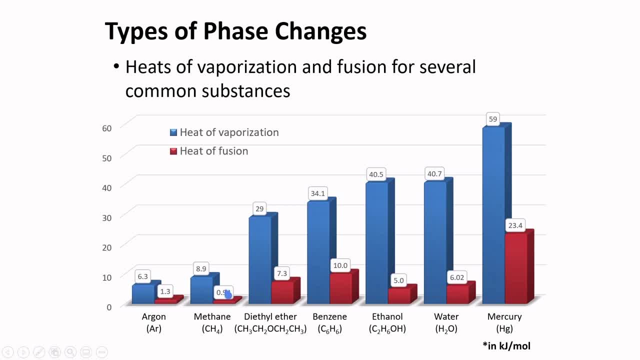 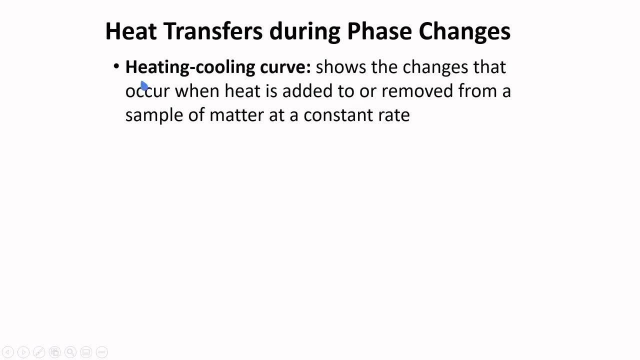 of fusion. it also shows the general increase of these enthalpy values as the strength of the intermolecular forces within these substances. Heat and cooling curves show the changes that occur when heat is added to or removed from a sample of matter at a constant rate. 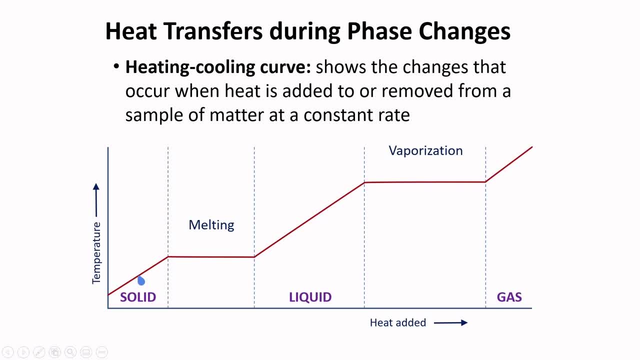 We can start from a solid and as heat is added to this solid the temperature will increase where liquid forms. Then, as heat is added further, we will get to a point where the liquid will start to vaporize and form the gas. Further infusion of heat will further 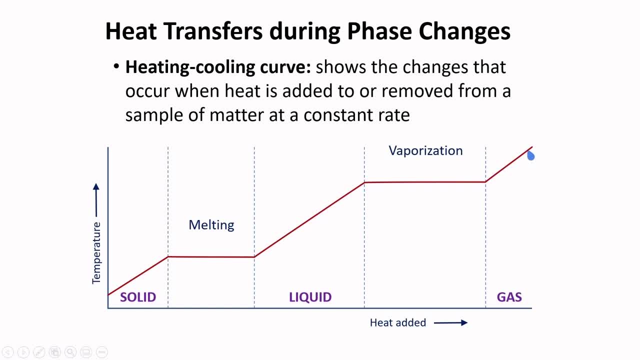 increase the temperature associated to the gas particles. Within a phase, the infusion of heat is accompanied by a change in temperature, and a phase change occurs at a constant temperature. The amount of heat involved in these transformations can be calculated using the following formulas. These are formulas that were discussed in 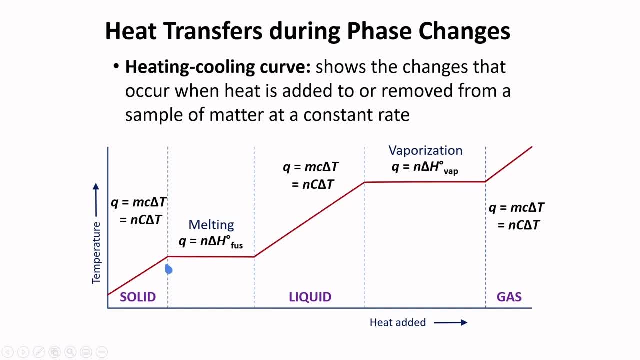 the thermochemistry topic. For example, In solids, heat can be calculated from the mass, specific heat capacity and change in temperature of the substance. The amount of heat involved in the phase change can be calculated using the molar heats of fusion and the molar heats of vaporization of the substance. 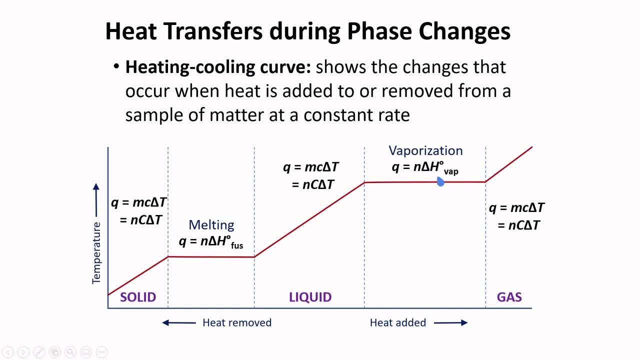 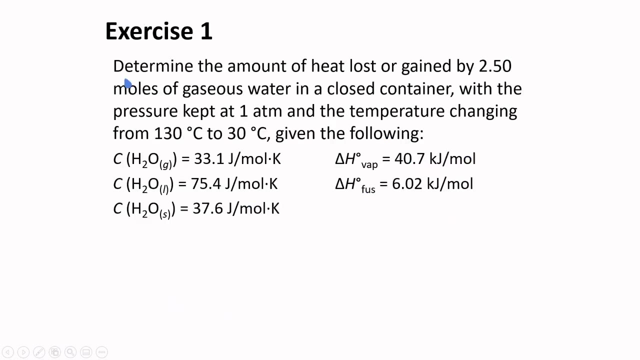 We can also calculate the reverse when heat is removed. For example, We can use was mean, as we appreciate that the amount of heat involved in gdzie is waterless denoted in bold, In this case With condensation and freezing, As mentioned in. 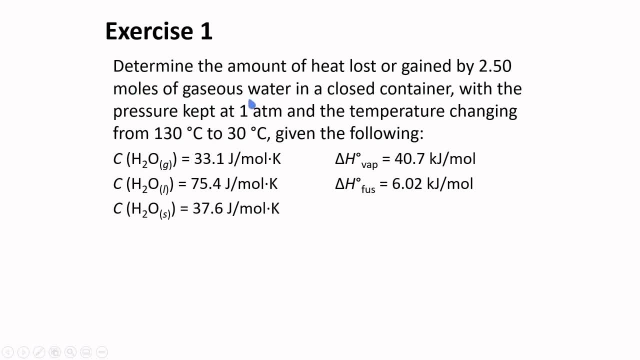 the previous slide. there is only a change in sign during this calculation Exercise. 1. Determine the amount of heat lost or gained of gaseous water in a closed container with the pressure kept at 1 atmosphere and the temperature changing from 130°C to 30°C. given the following values: 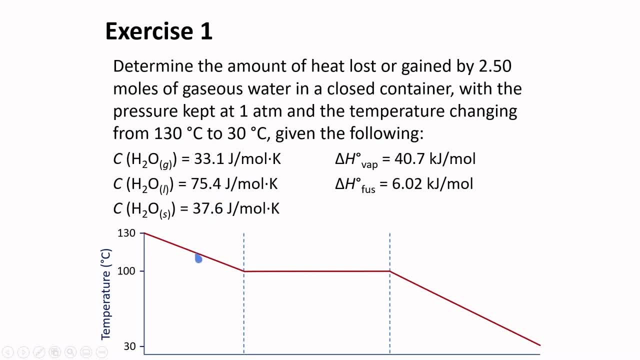 We could illustrate this change using this cooling curve. The starting temperature is at 130°C. Here, only water vapor is present. As heat is removed from the system, the temperature will cool down to 100°C. Here the temperature will remain constant until all the water vapor is converted to liquid. 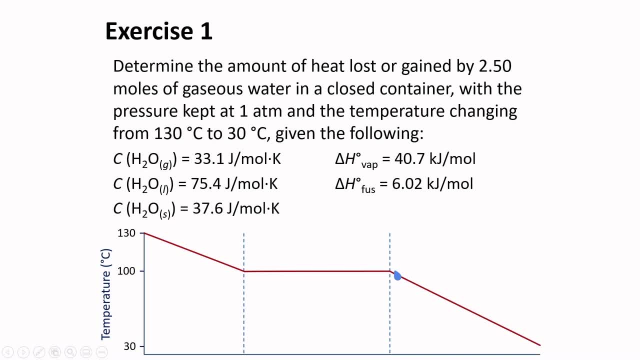 When this transformation is completed, the temperature will go down again until the final temperature of 30°C is reached. Thus we can have three stages. In stage 1, we can use the molar heat capacity of water vapor. In stage 2, the molar heat of vaporization is employed. 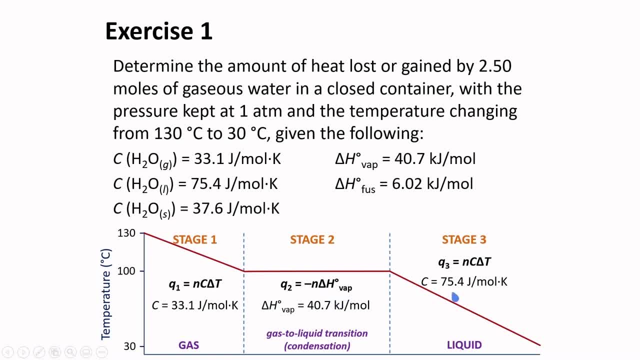 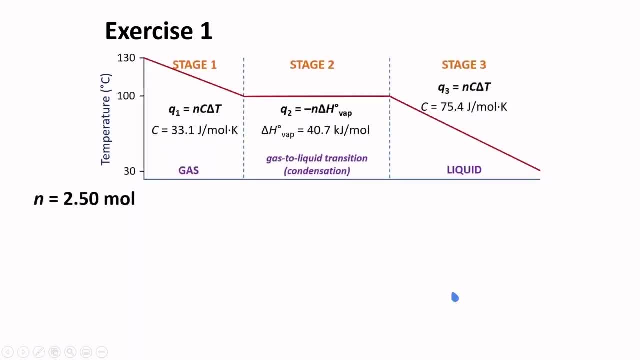 And in stage 3, we can use the molar heat of vaporization. In stage 4, the molar heat capacity of liquid water is utilized. Take note that 2.50 moles of water is present For stage 1,. we first need to calculate the change in temperature. 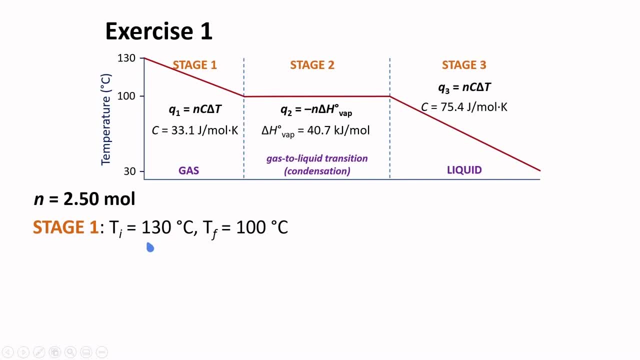 Given that the initial temperature is 130°C and the final temperature is 100°C, delta T is equal to negative 30°C. The unit degrees Celsius needs to be converted to the Kelvin scale for consistency, And in this case we can have the same numerical value for the change in temperature, negative 30 Kelvin. 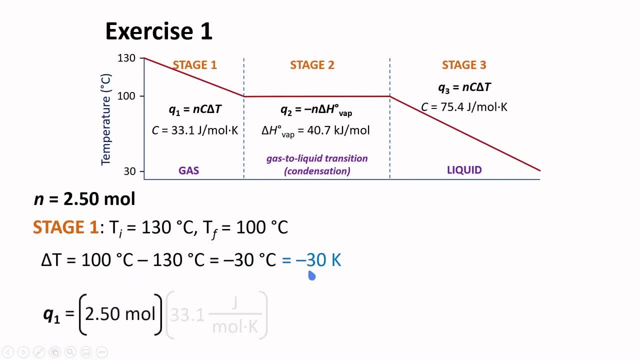 Logging in these values to the formula and canceling the units. Q1 is equal to negative 2,500 J or negative 2.5 kJ. For stage 2, this occurs at a temperature of 100°C. Here the values are just plugged in to the formula. 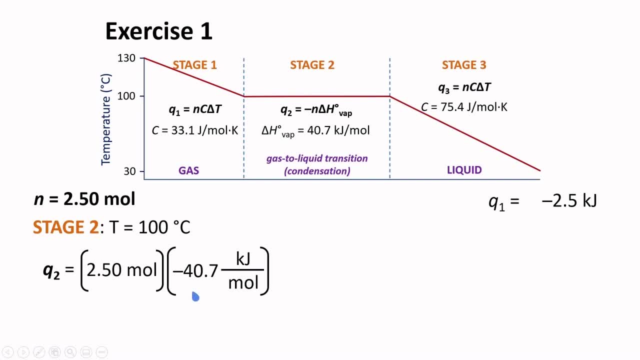 The heat of vaporization is given a negative value. This is equivalent to the molar heat of condensation at 100°C. Moles are cancelled And we will get negative 2,500 J. We will get negative 102 kJ. 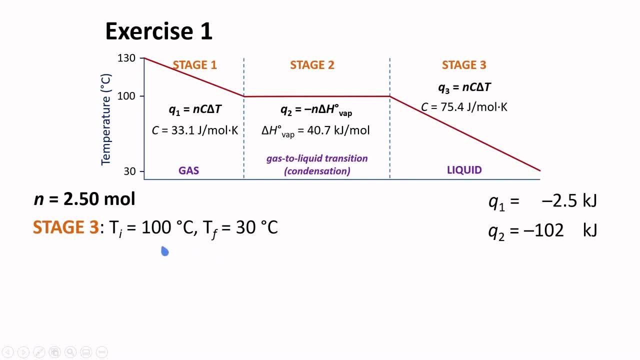 At the last stage, stage 3,, the initial temperature is 100°C And the final temperature is 30°C. Our delta T is 30 minus 100°C is equal to negative 70°C. We convert this value to Kelvin, this value to Kelvin, and take the difference. 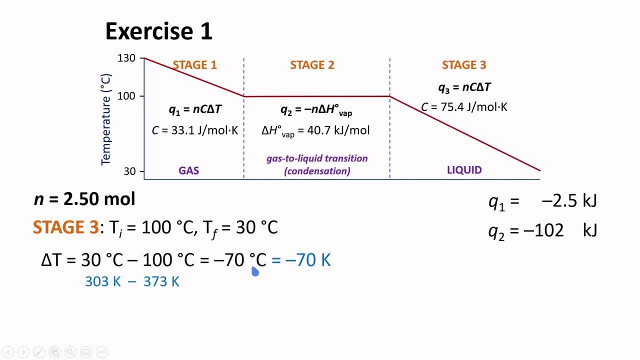 And the numerical value in Kelvin is equal to the numerical value in Celsius. If we plug in to the formula, we will get negative 13,000 J or negative 13 kJ, Taking the total of all the heat values for stage 1,, 2, and 3,. 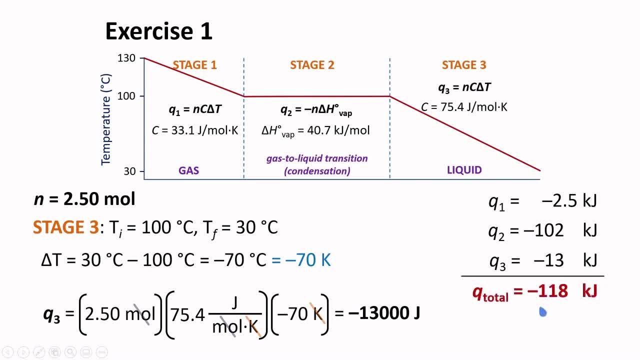 we will get negative 118 kJ. It means that 118 kJ is lost by the system during the whole process. Thank you for watching.